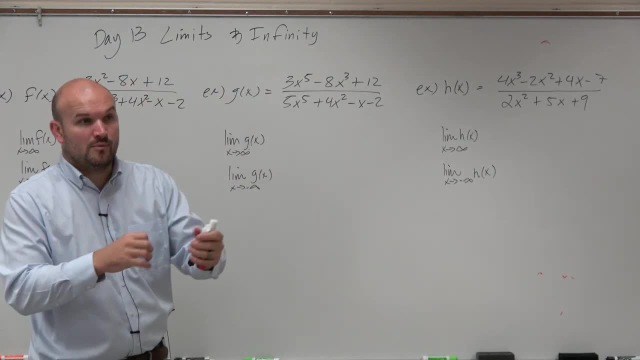 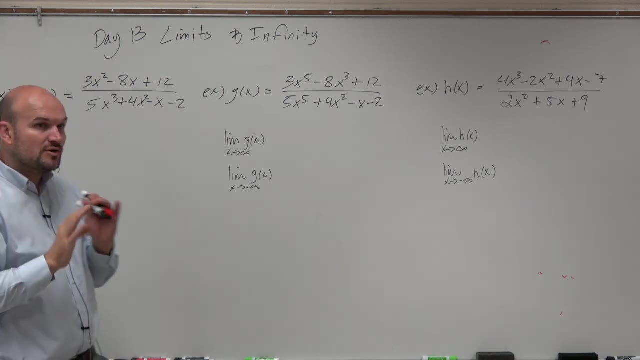 Or we're getting into more difficult ones later when we're dealing with different types of functions. But when we're dealing with rational functions, polynomial in the top and the bottom, our most important thing is we want to do is identify the asymptotes. 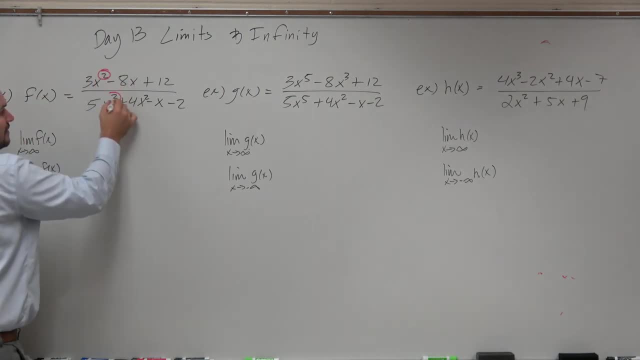 So again, remember what I did, is you know? I looked at, compare the degrees in the numerator and the denominator And here the degree in the numerator is less than the degree in the denominator, Correct Right. So 2, obviously is less than 3.. 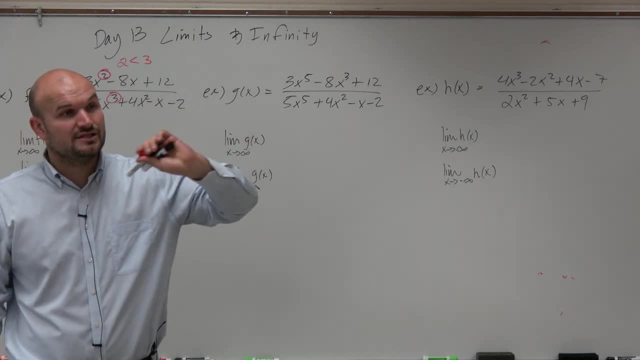 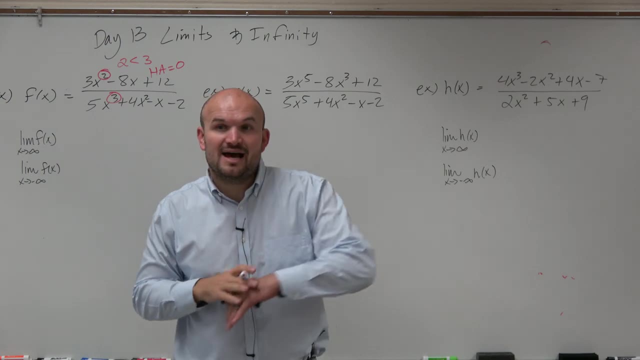 So, if you guys remember, when the degree in the numerator was less than the degree the denominator, the horizontal asymptote was equal to 0.. So it doesn't matter, as the graph is going towards infinity or going to negative infinity. 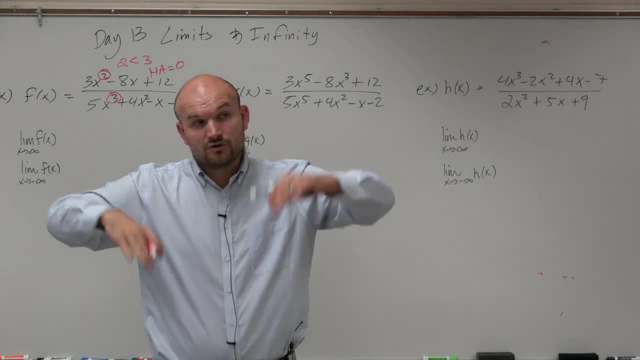 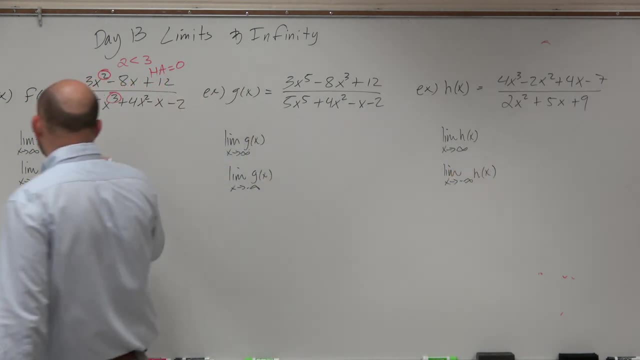 It doesn't even matter what the graph looks like. We know that the graph, it can cross the horizontal asymptote. it can do all this stuff, But we know its end behavior is going to be approaching the horizontal asymptote. So the first one: doesn't matter if it's infinity or negative infinity. 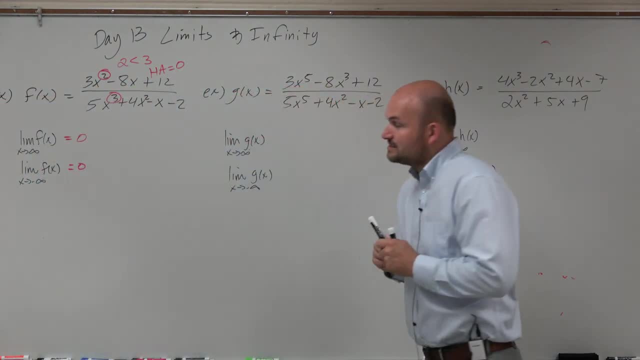 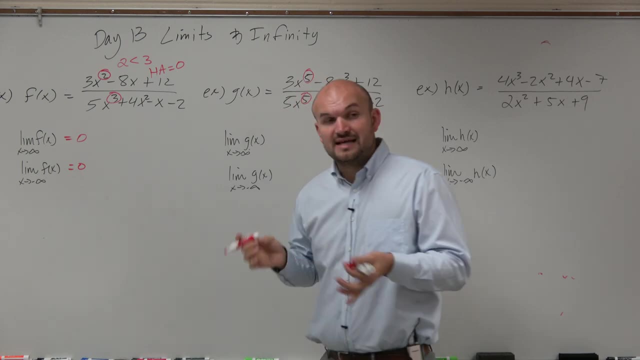 It's going to 0.. Done, Move on. Okay, So the next one is: again, we're identifying the degrees of them, 5 and 5.. Since the degrees are exactly the same in the numerator and the denominator, 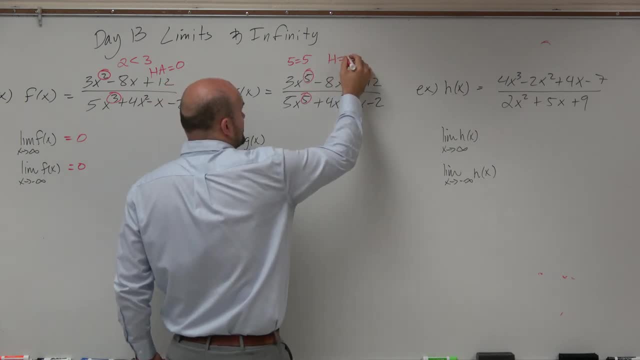 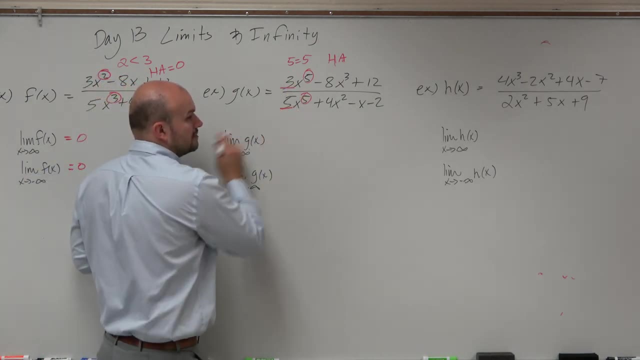 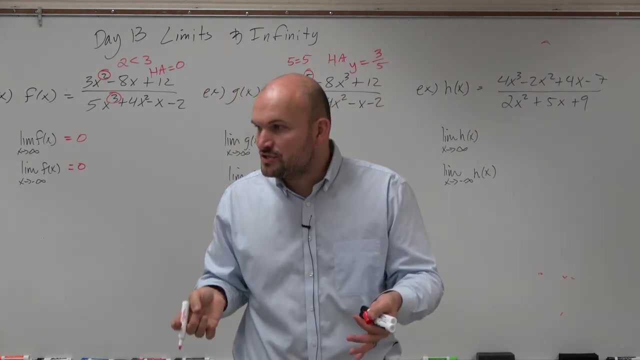 we know that the horizontal asymptote is equal to the ratio of my coefficients. So my horizontal asymptote is: y equals 3 fifths. Again, it's an asymptote. So the graph- no matter who cares what it looks like. 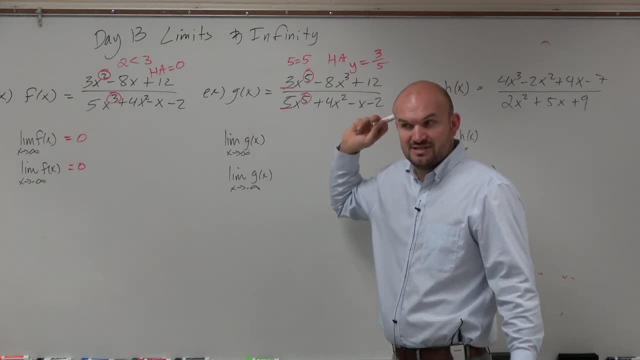 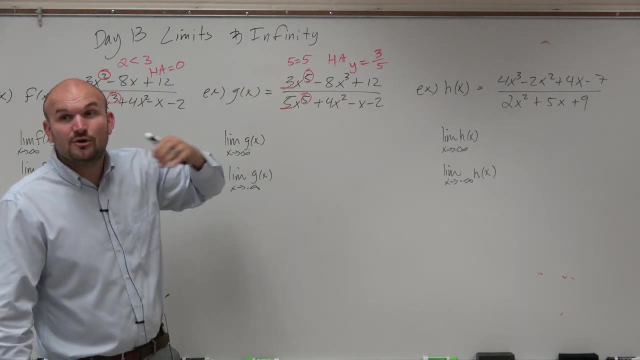 who cares what all the rest of the function is or the polynomial is, it doesn't matter. We could put fractions and decimals and make it look all crazy, but it's still. in the end it's a polynomial. It's going to approach its horizontal asymptote. 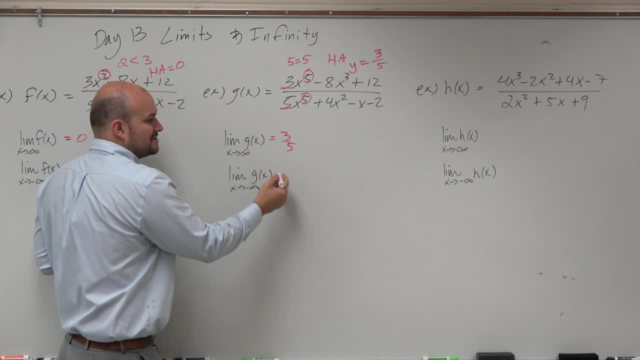 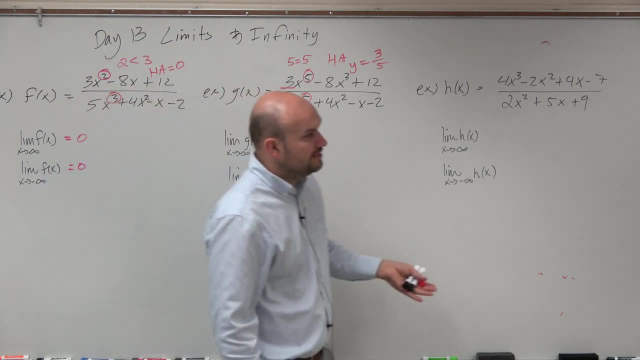 As it goes to infinity- 3 fifths. As it goes to negative infinity- 3 fifths Done. Now, in this last one we have a little bit of an issue Because the graph has now What we have is a horizontal or, I'm sorry, a slant, or an oblique asymptote. 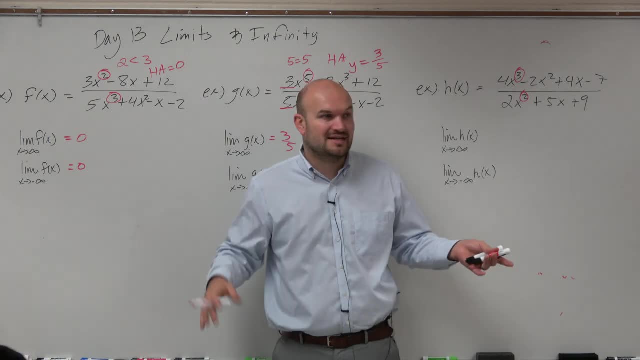 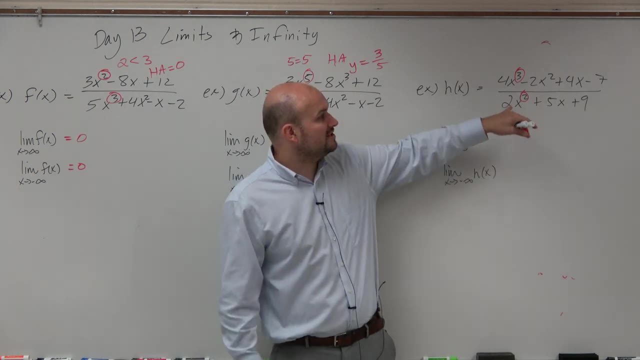 So our first thing I showed you was like this long way of making sense of it, We could do long division. Nobody is going to want to do long division, Right, So we can just mark that out. The next one was: but in reality, when you do do long division,